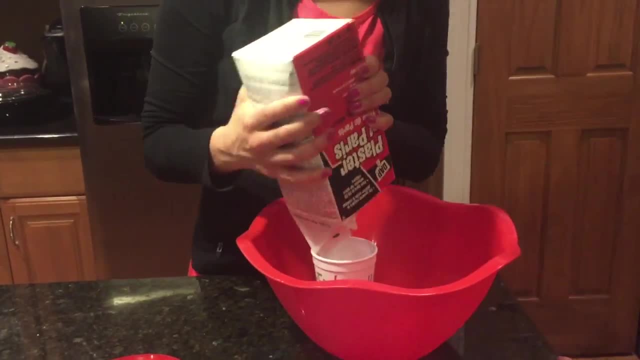 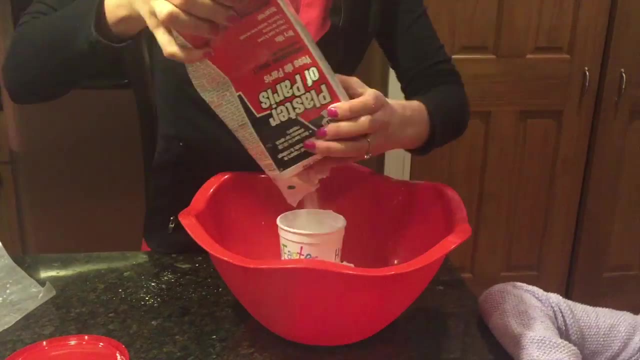 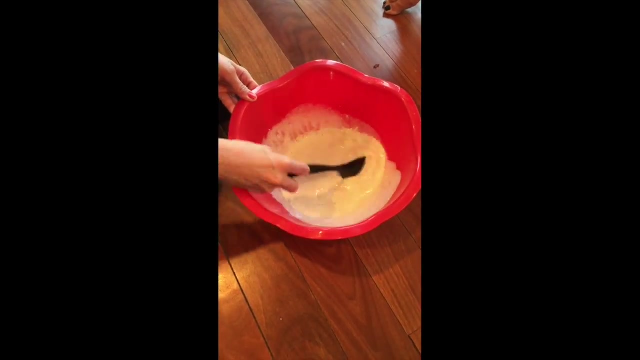 so now you're ready to make the plaster of paris. the directions say two parts plaster, one part cold water. this is about a 10 ounce cup. it was more than enough to make three molds. so i put two cups of the plaster, one cup cold water and i mixed it until it was creamy and smooth. 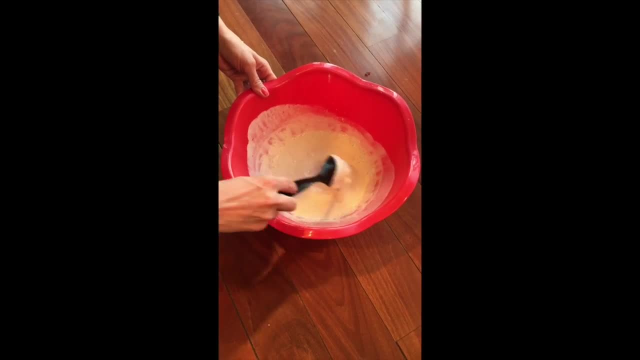 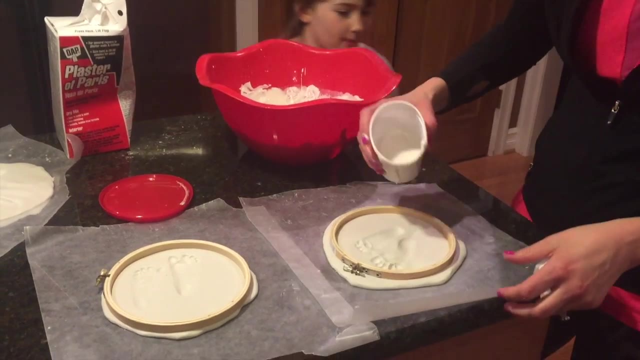 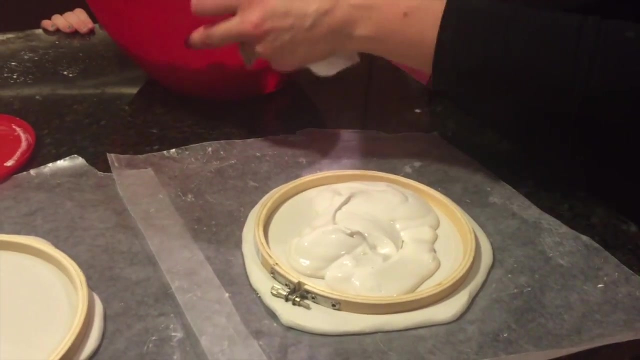 and once it's mixed pretty, pretty well, you're going to want to take your cup and pour it right on top of your prints, and don't be afraid to just get right in there. get a nice smooth coat over the top. it's not going to go on smooth actually, to begin with. 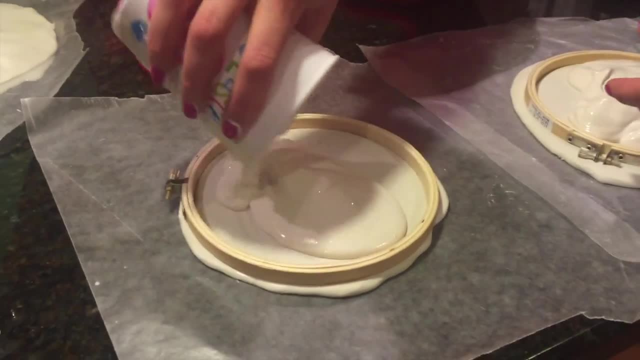 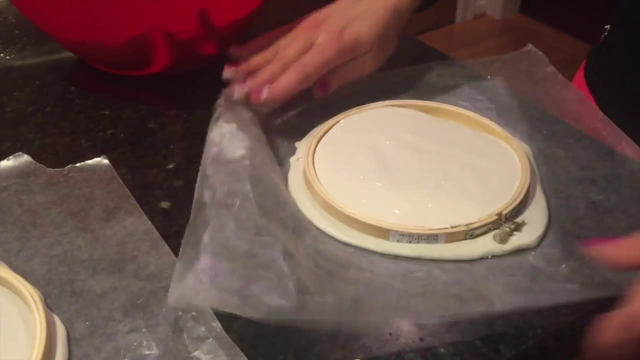 or even i should say, but just pour it on there. you want to make sure you don't overfill the ring. if it looks like you could add a little more, just use sparingly. you don't want it to spill over and then just take the wax paper. 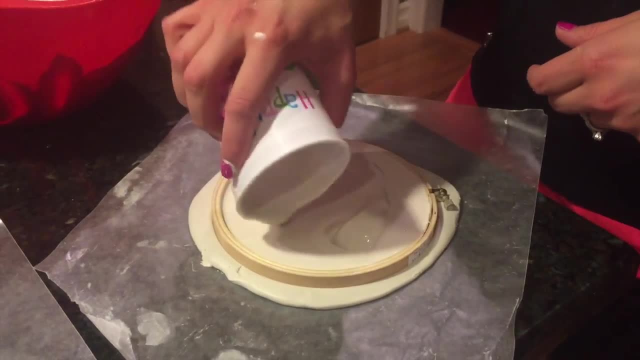 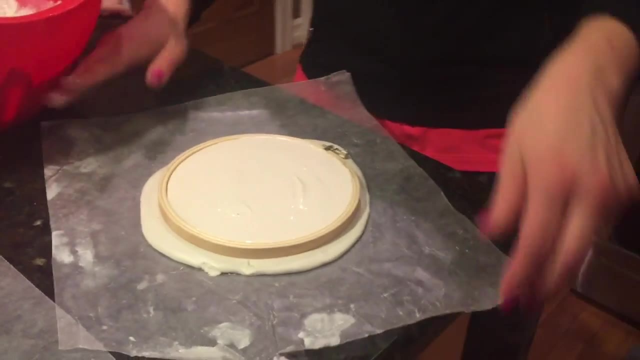 and wiggle it. don't use a spoon to smooth it on top. just use your hands on the wax paper and give it a good, a good shake. the most important part about this process is to make sure that you pound your fist around the mold. you'll see the 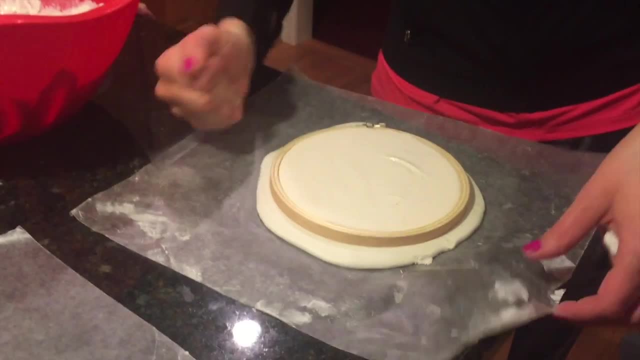 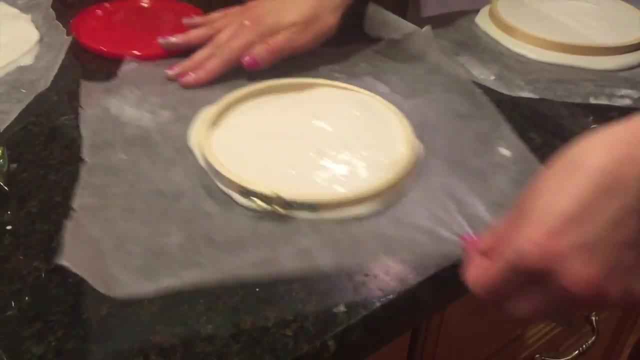 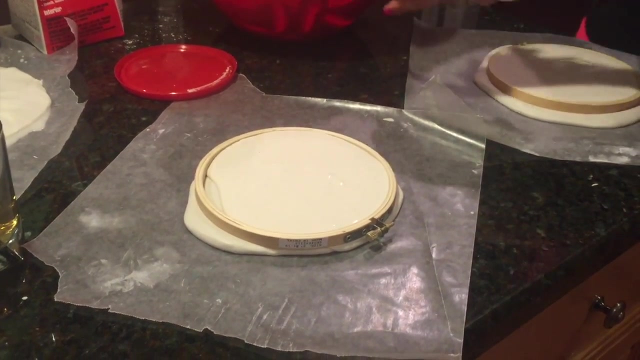 bubbles popping. if you don't do this, you will get bubbles on your mold and it it ruins the project. it really doesn't look good. so make sure that you're doing this on a hard surface and just pound about I don't know 10 times or so around. 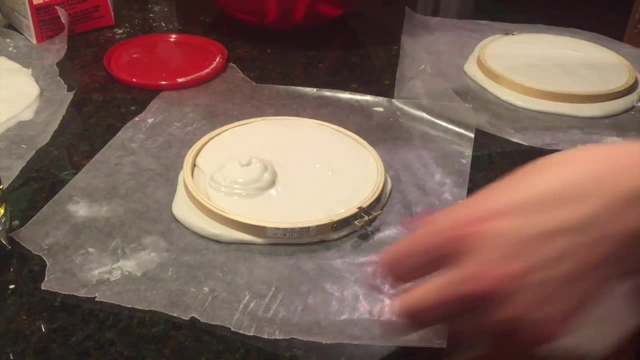 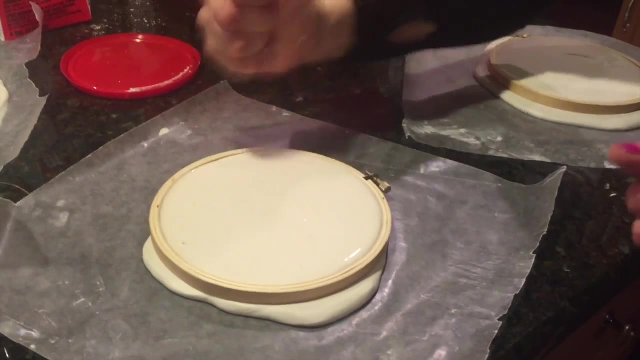 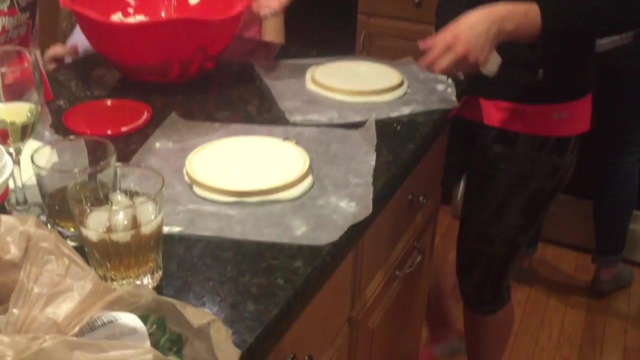 the mold and you'll see the bubbles popping through and that's how you know you're getting them all. I have an example of a mold that I didn't pound on, so this might be a little tricky. it's very, very difficult if you're not pound. I was actually doing the mold on a glass table, so I was nervous to to break. 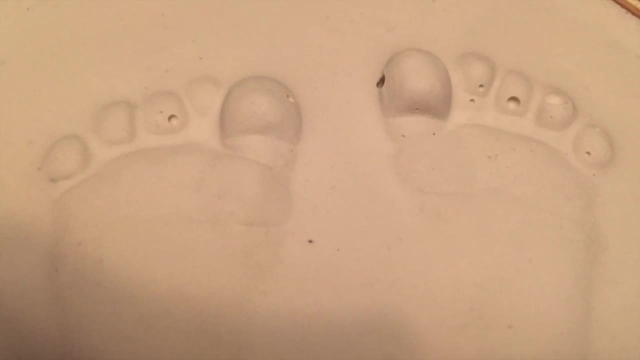 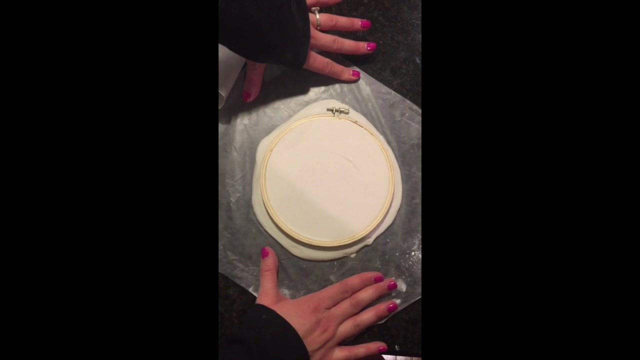 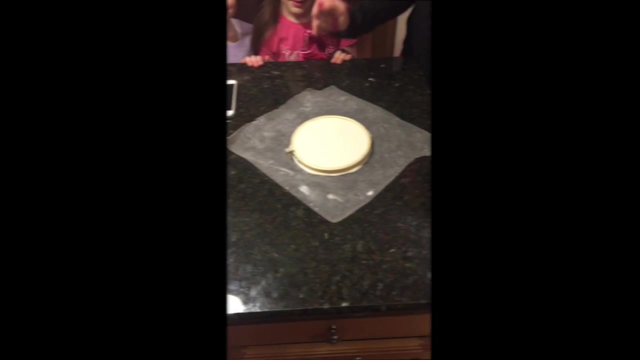 it and the toes came out pretty bad. so this is what you don't want to check to make sure whether your mold is ready. you just want to shake the wax paper. if you see it still wiggling, it's not ready. you'll know when it's hard it will feel.